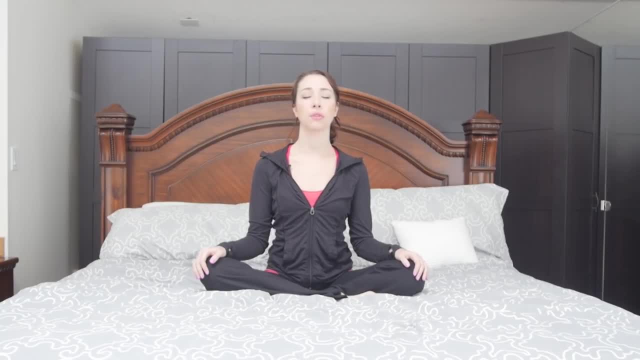 four. where you inhale for a count of four, you hold that breath in for a count of four and you exhale either for that same count of four or maybe for a count of eight. so the act of holding the breath and lengthening the exhale helps to activate the parasympathetic nervous system. 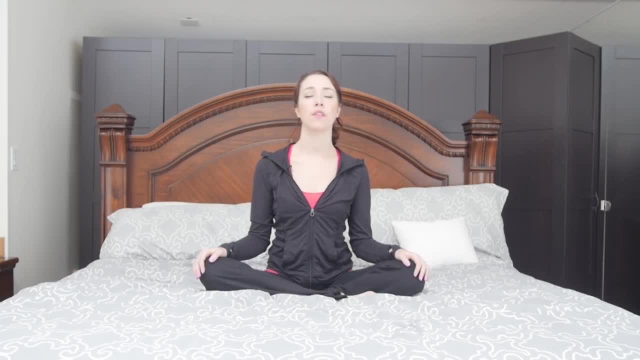 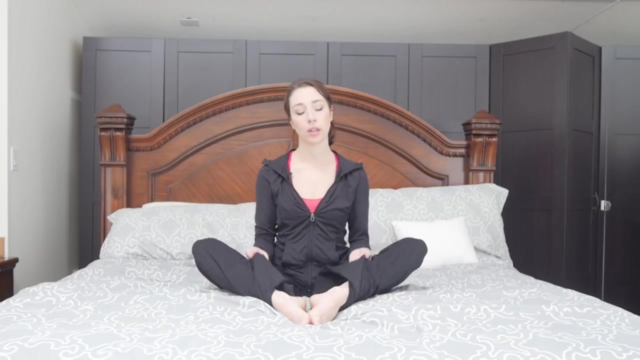 and helps to relieve anxiety and facilitate a good night's sleep. so you're welcome to maintain this breath. we'll come into a butterfly fold. just bring your feet out in front of you, soles of the feet together, knees apart, and we're really not trying to push ourselves in this one, so get as comfortable as you can as you fold on down. 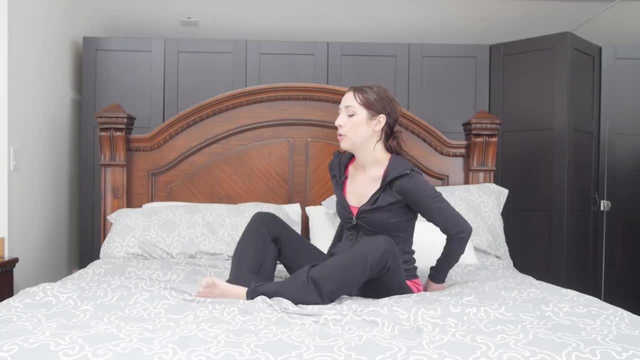 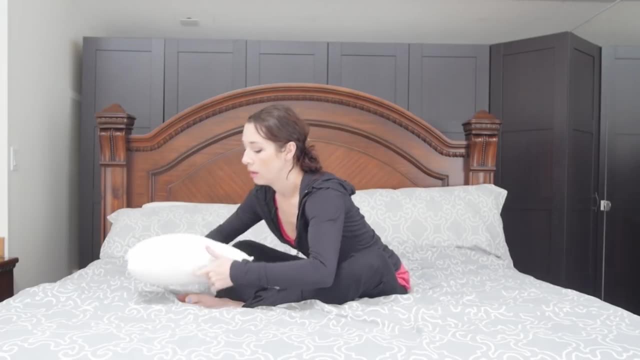 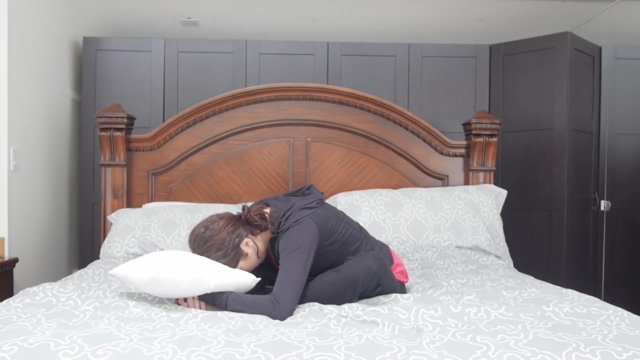 i'll just turn to the side a little bit. you're welcome to use your pillows as cushion underneath the forehead or underneath the chest, just getting nice and comfortable. you can turn one ear to the pillow or you can just let your forehead come down and, once you settle in this first pose, find that breath rhythm. 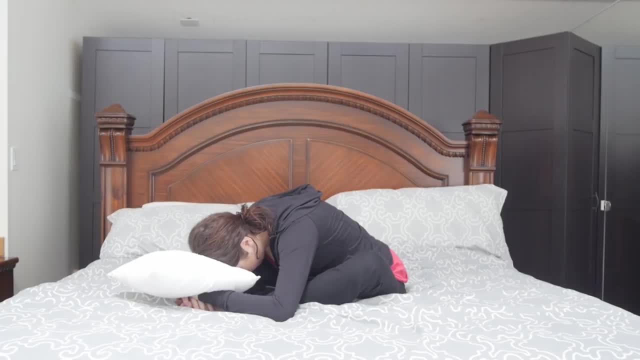 either four four, four or four four, four or four four, four, four, eights. whenever you notice your mind start to wander, just bring it back to the present moment, focusing on your breath. imagine the tension melting out of the shoulders, pouring out the crown of your head. take your last five breaths here. 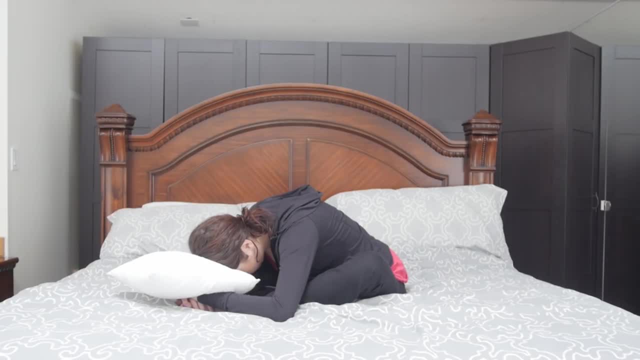 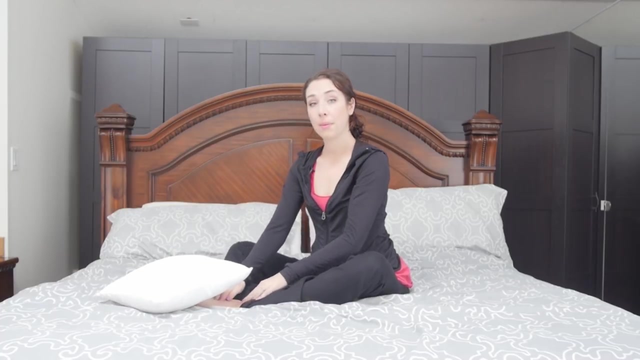 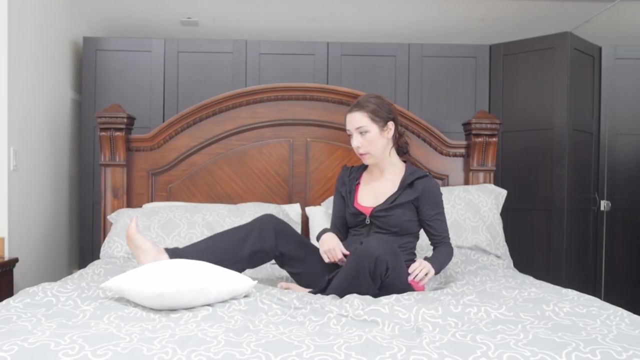 and very slowly ease your way out, unwinding. we'll come into another forward fold. forward folds are really the best kinds of poses that you can do before bed- really great stress relieving poses. so you can extend your right leg out in front of you, bring your left foot. 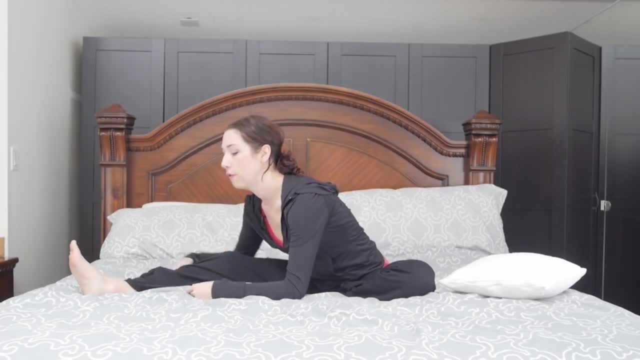 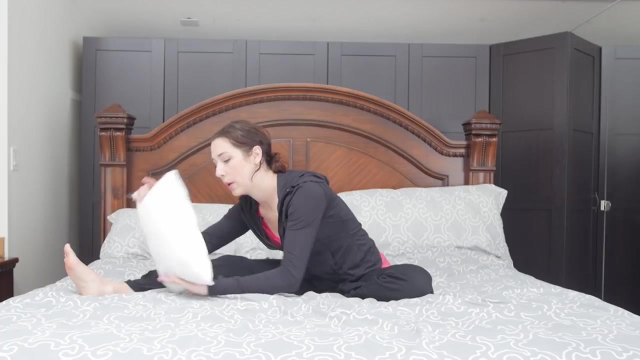 to the inside of that thigh and we're just going to fold ourselves over that right leg and dangling is perfectly fine here. you don't need to be supported with blocks or pillows or anything like that. you can just let gravity do the work for you. but if you're somewhere close, you can always. 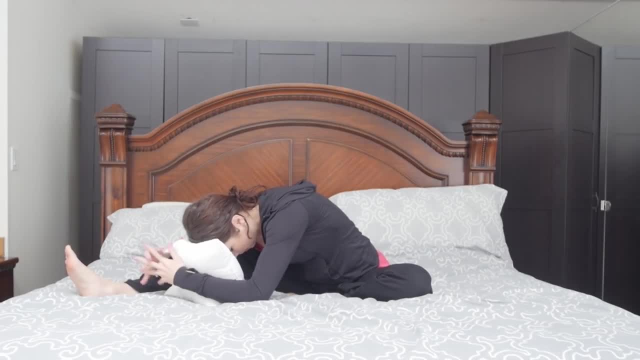 just close that gap with a little pillow. the mattress is great because it allows our knees to stay a little bit bent, which is what we want. we're not chasing sensation here. we're not trying to push ourselves into any kind of pose. this is really just to relieve. 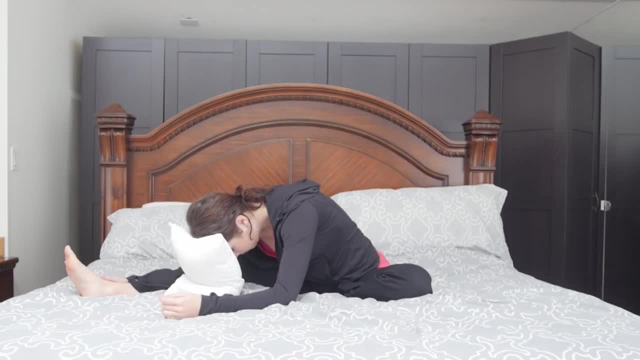 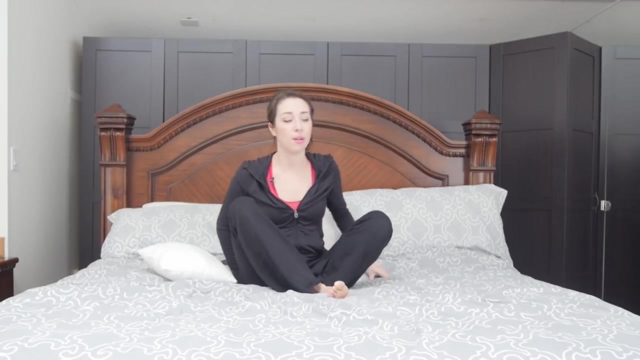 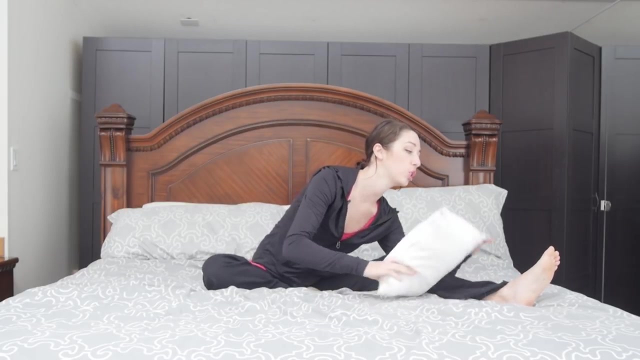 ourselves of any aches and pains so that we can ease into a great night's rest, you, and come on up and move to the other side so you can bring your right foot in and extend your left leg out and folding over, this time towards the left foot, towards the left shin. 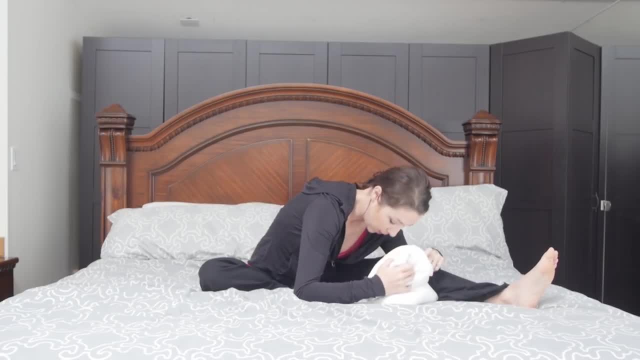 maybe propping yourself up with a couple pillows, or just dangling and letting gravity do the work for you here. relax your arms by your sides and ask yourself to relax and hold your breath for a few seconds, and this is the best way to do this. so, now that we've had this session, it's time we're going to go back to our 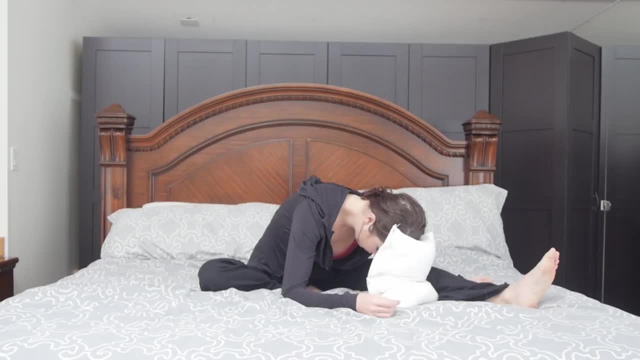 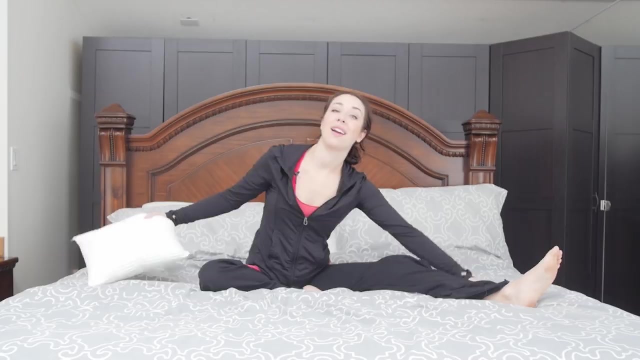 buttocks. stay relaxed and relax and go ahead and relax, Soften your shoulders and your upper back And start to lift back up. Now we're going to lie all the way down, so I'm going to turn to the side, just so it's. 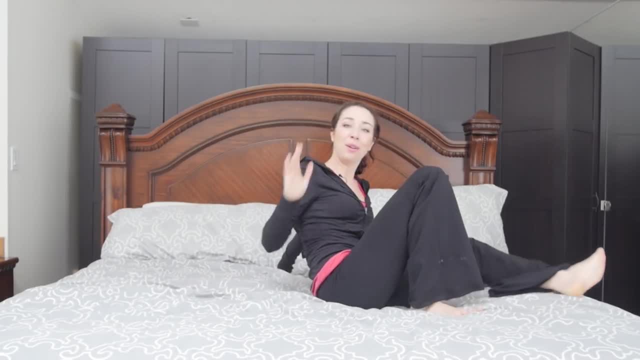 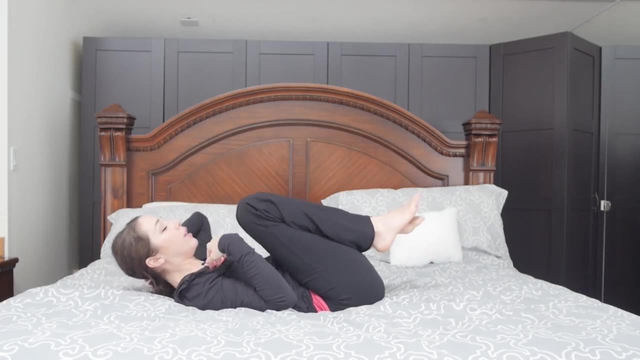 easier for you. I'm going to show you guys to see what I'm doing. But you can lay right down the way you normally would And just pull your knees into your belly, giving it a big squeeze, maybe rocking a little bit side to side, massaging the low back. 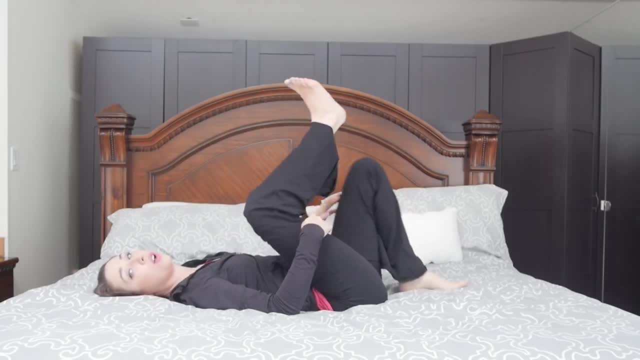 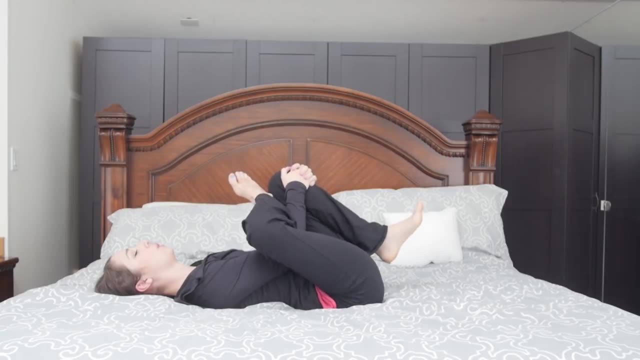 And we'll come into reclined pigeon pose so you can cross your right ankle over the top of your left knee And maybe, staying here, you can reach through with your arms and pull that left knee into the belly, Just inviting that glute to relax, to open up. 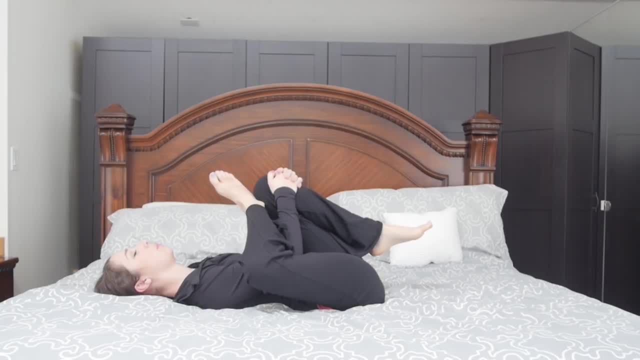 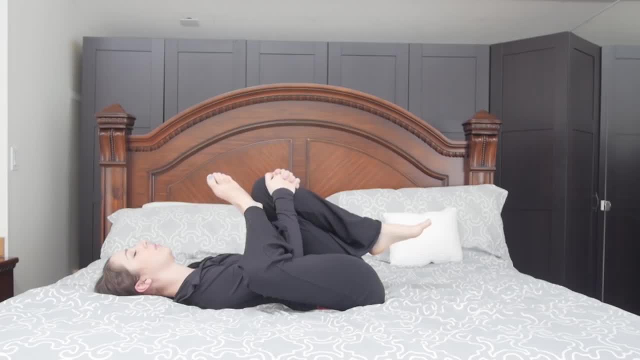 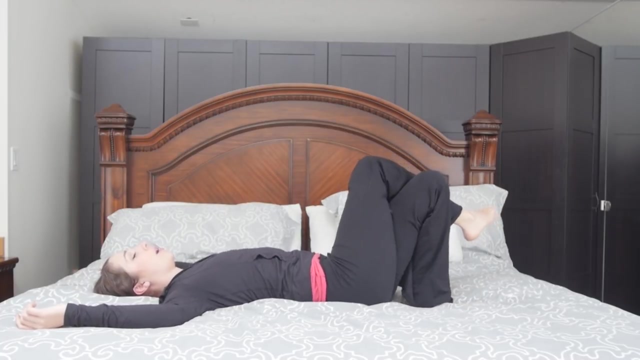 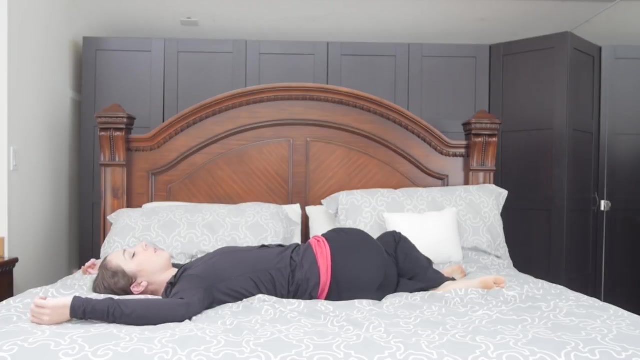 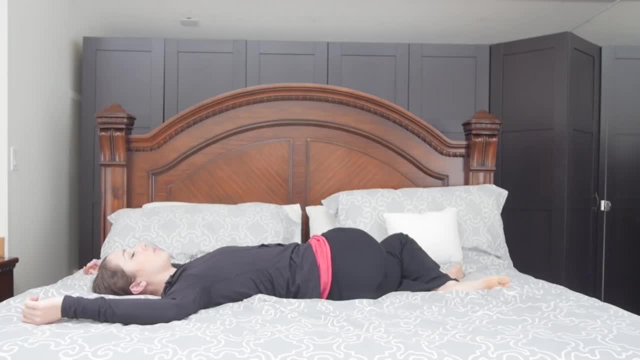 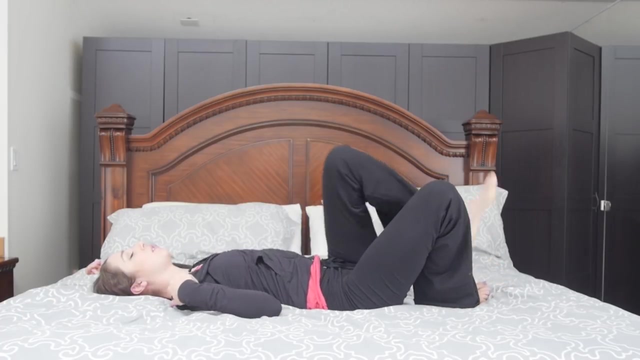 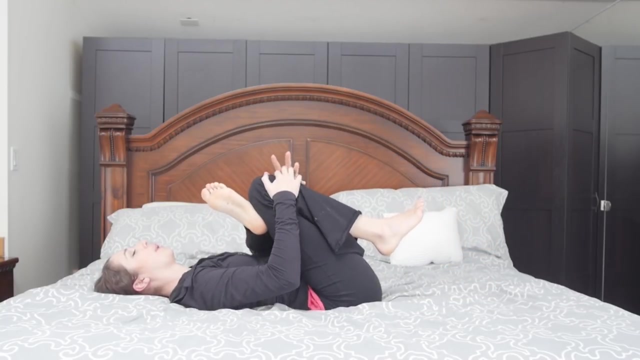 low back And release Both legs. come back up Reclined pigeon on the other side, left ankle crosses over the top of your right thigh And you can pull through with your arms, drawing your legs back up And bring your right knee into your belly. 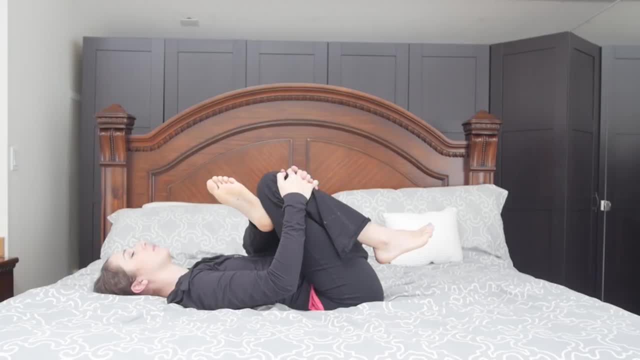 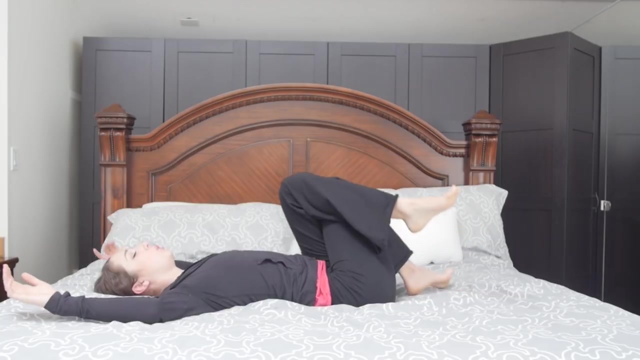 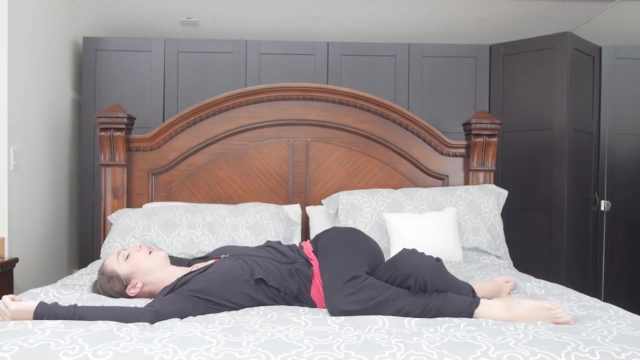 And one more big squeeze And come to your twist on the other side. Wrap your left thigh over your right, Reach your arms out to the sides And your hips might need to move to the left before both knees come back up And just drop down over to the right. 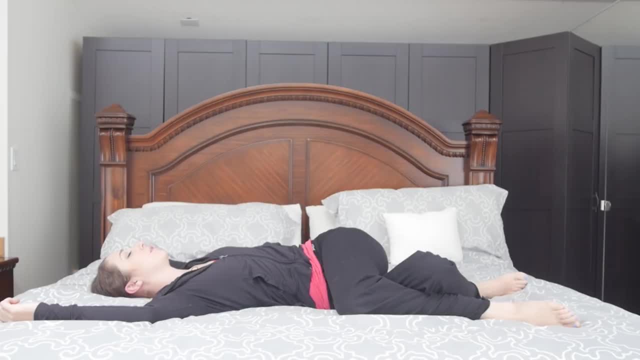 Continue to breathe down deep into your belly, Deep into the low back. And one more big squeeze yarn over. draw two super long tenho by�� игi. three by죠 bydy ragol does. Who will we learn more about? 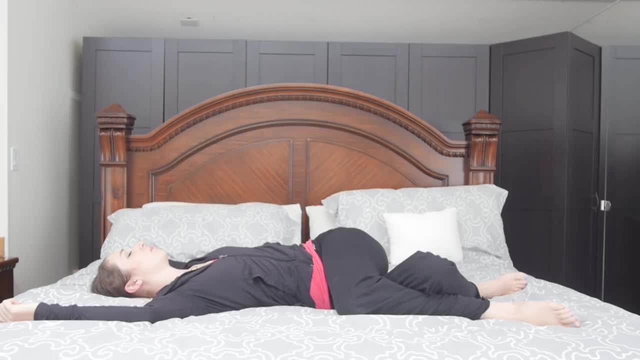 How to do. who is the cook? How do you give birth to your child? Do you give birth to your baby? Most of the time, they should be alive. That is very helpful. Do you need to fully meme vive? You land up a fat. you get birthed out. 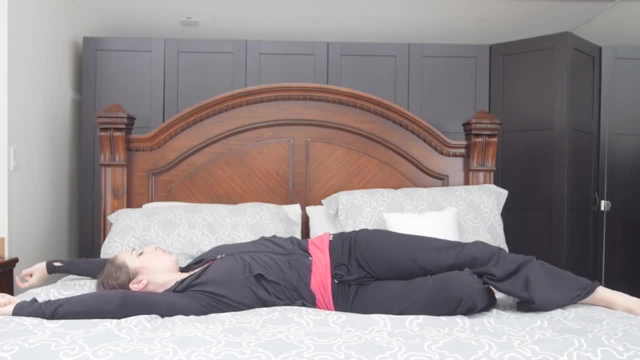 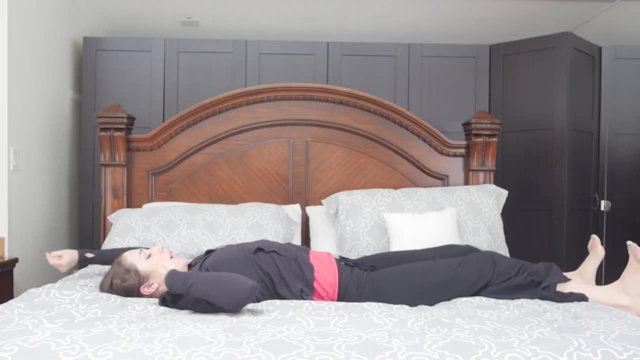 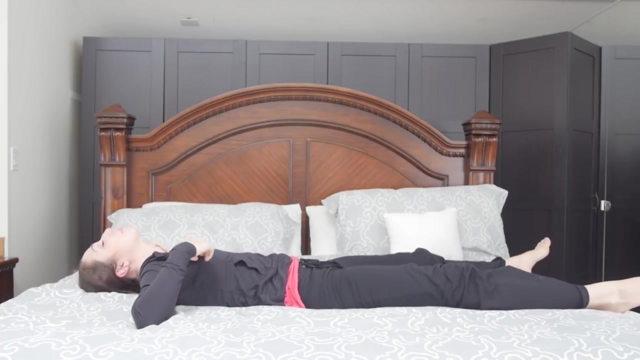 Maybe can you know anything new on Tinder. Now, how do you know, Of course, how to do that? you can take a big stretch, reach your arms up overhead, straighten your legs, go ahead and get yourself under the covers. I'm just gonna stay as I am here taking. 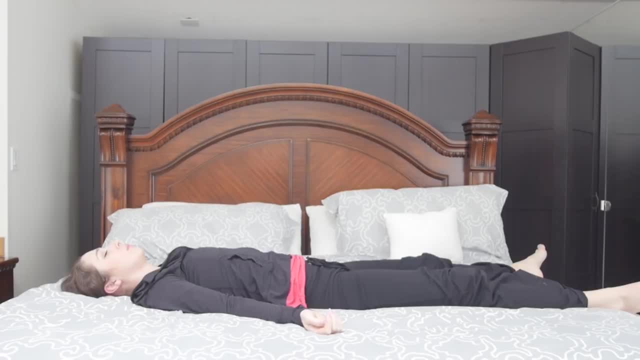 shavasana. you just notice if there are any lingering aches and pains, any points of tension. if you need to do any other little movements, you're welcome to come into it here. but we'll finish with a bit of a body scan, like a body relaxation meditation, and then the video will. 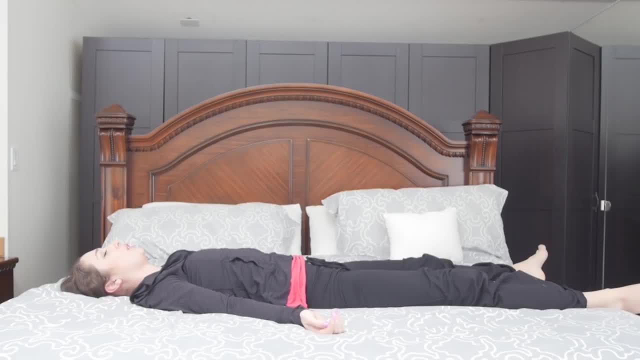 gradually come to an end and hopefully you'll be ready for sleep. so take up space palms facing up to the sky, close your eyes and, just internally, bring your awareness to the crown of your head, moving your way down and relaxing the forehead muscles along the eyes, the cheeks. 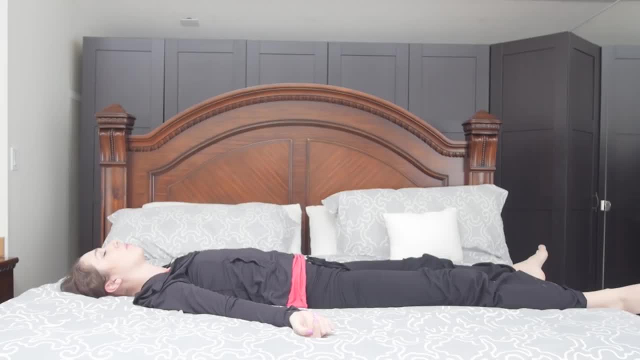 the tongue, the neck and jaw. Focus on your right shoulder and invite it to relax Down into the right upper arm, right elbow, right forearm, right hand and fingers. Feel your right arm completely relaxed and heavy And then over to your left shoulder- left shoulder. 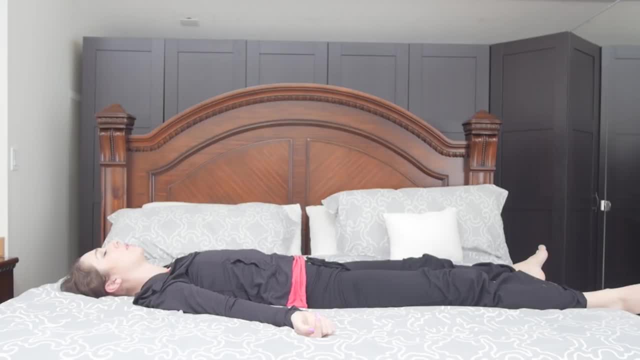 left upper arm and elbow, left forearm, hand and wrist. Relax your left arm completely. Bring your awareness to the chest and the upper back, the belly and the mid-body Down into the pelvis, into your lower back and into your hips. 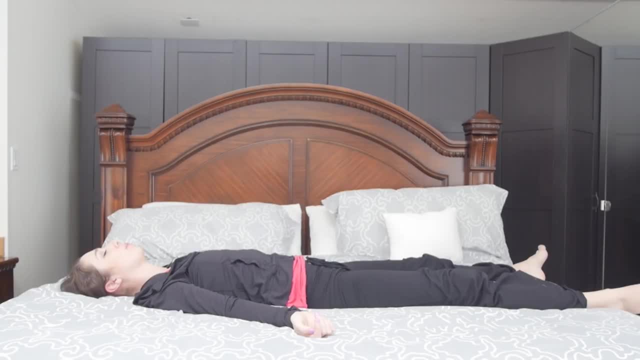 Feel them get heavier, with your breath Sinking deep into the mattress underneath you. Focus on your right glute, your right hip, right quads and right hamstrings, Softening down into your right knee, the right calf and shin, into your ankle, your toes, the sole of the foot. 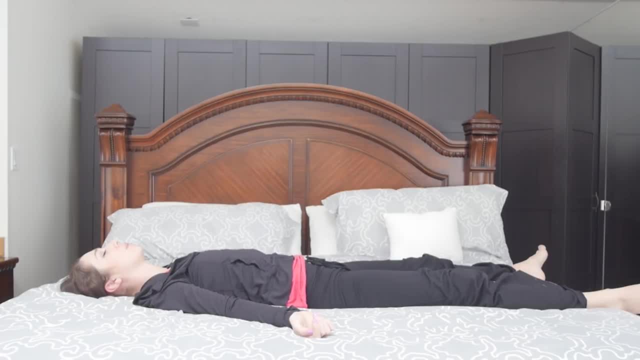 Observe your right leg, completely relaxed. Focus now on the left hip, the left knee, the hi farewell leg- hamstrings and hamstrings. Relax agus halfway The thigh, the hamstrings, the hamstrings, the upper elbows your higher, lower colocablia. 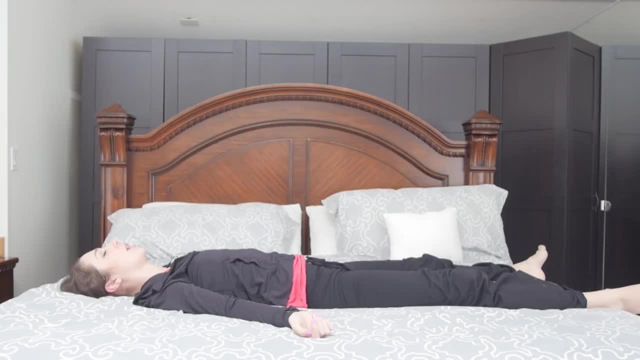 clavicle your collarbone, the hamstrings and the hamstrings. Relax your left knee. Relax your left knee. Bend your, baker yourselves The리 into the ankle, the heel, the toes, the sole of the foot. Soften your left leg and observe your body as a whole. 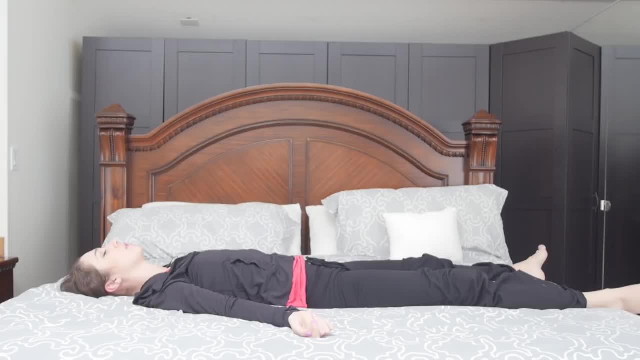 Melting further into the mattress, releasing more tension with every exhale, Letting your thoughts wander a little bit so it can turn into a dream as you drift off. And this is where I will leave you, yogis. Have a wonderful night, namaste.